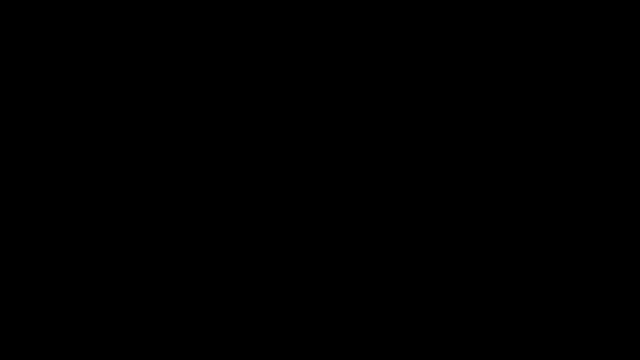 In this video we're going to talk about how to convert a percentage into a decimal. So let's start with this example: 75%. How can we convert this number into a decimal? A simple way is to divide 75 by 100.. 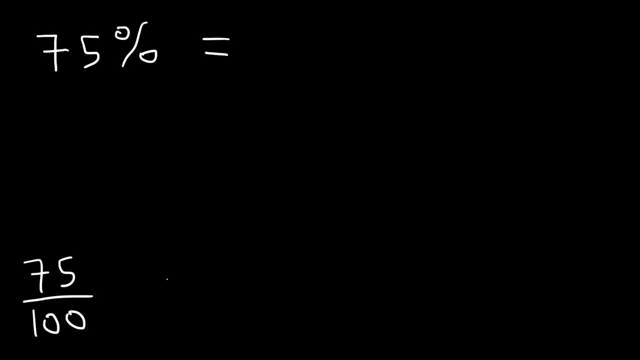 If you type this in your calculator: 75 divided by 100, this will give you .75 as a decimal. Or you can start with a decimal and move it two spaces to the left. So 75% is .75.. So let's try another example: 28%. 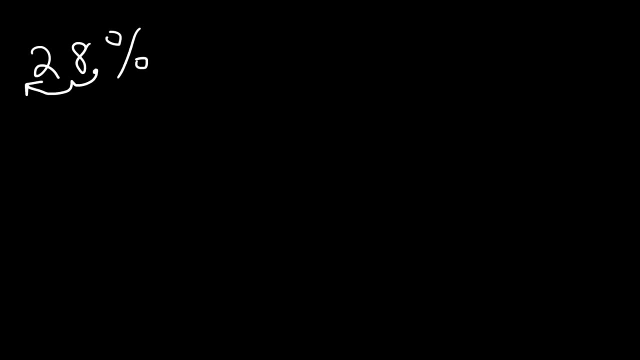 If we take the decimal point, move it two spaces towards the left or divide it by 100, this will equate to .28.. So 28% is .28.. Try this. Try these two examples. Convert 36% and 45% into a decimal. 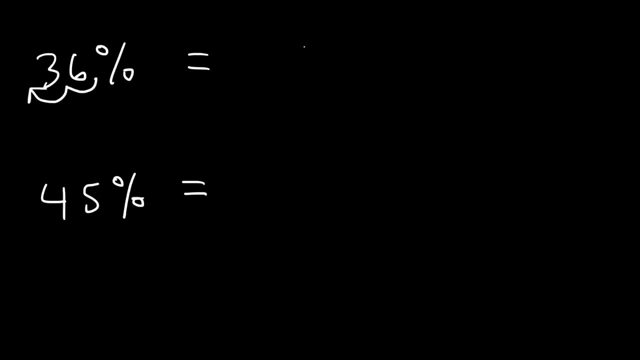 So if we move the decimal point two spaces to the left, this is equal to .36.. And 45% doing the same thing is .45.. Now what about 9%, 9%? What is the value of 9% as a decimal? 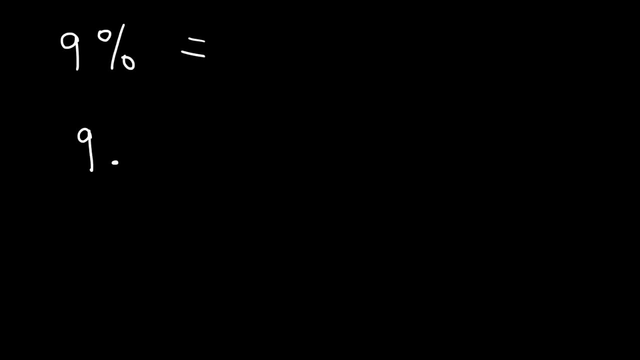 So if you start with the number 9, and if you move the decimal one, two spaces- which it should be here now- you need to add a 0. This will give you .09.. Now, what about 4%? What's the value of 4% as a decimal? 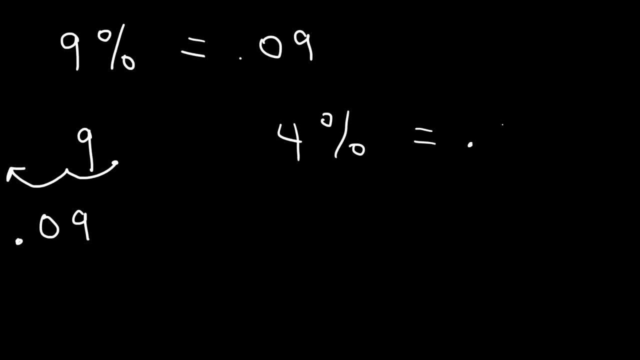 If 9% is .09,, then 4% must be .04.. Now feel free to pause the video and try this again. Convert 3.6%, 5.2% and 1.9% into a decimal for the sake of practice. 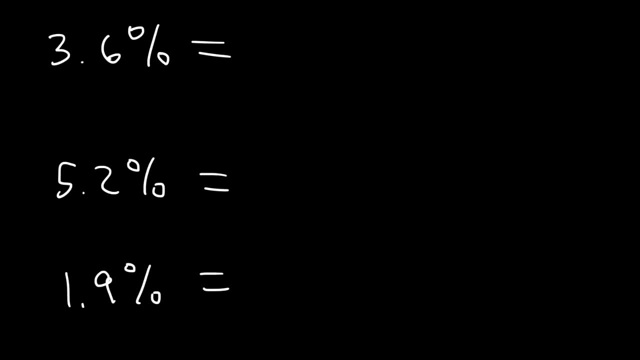 So if 4% is .04,, 3.6% must be .036.. Divide it by 100, or move the decimal two units to the left, So 5.2% must be .052.. And 1.9% is .019.. 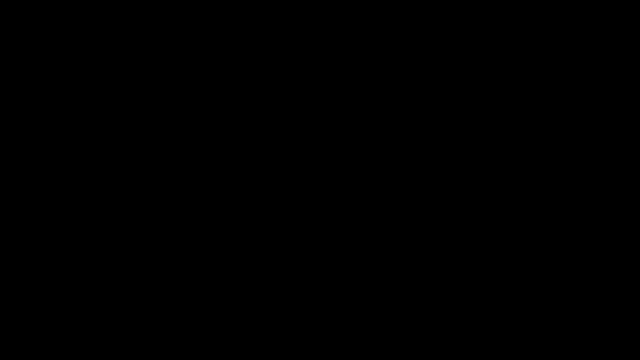 Now, sometimes you may have a percentage that's larger than 100. So what is the decimal value of 136%? So if we take the decimal point and move it two units to the left, it's going to be between the 1 and the 3.. 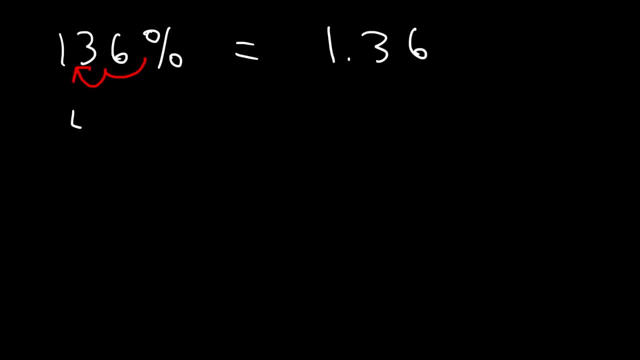 So this equates to 1.36.. So, based on that example, convert these values Into a decimal. So if 136% is 1.36,, 438% must be 4.38.. 596% is 5.96.. 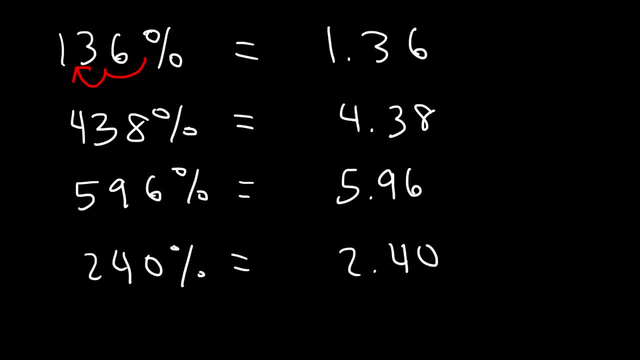 And 240% is 2.40, or simply 2.4. You can write it both ways. Now, in other cases, you may have a number that's less than 1.. For example, let's say if you wanted to convert .15% into a decimal. 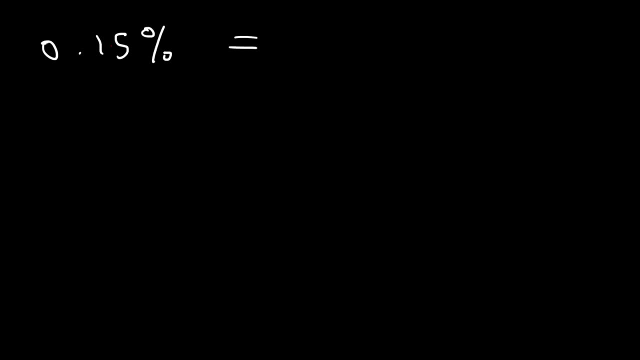 You want to follow the same pattern, Move the decimal point two units to the left, Or simply take a calculator type in .15 and then divide it by 100.. So .15 divided by 100 is .00.. If you move it two spaces to the left, this is 1, this is 2.. 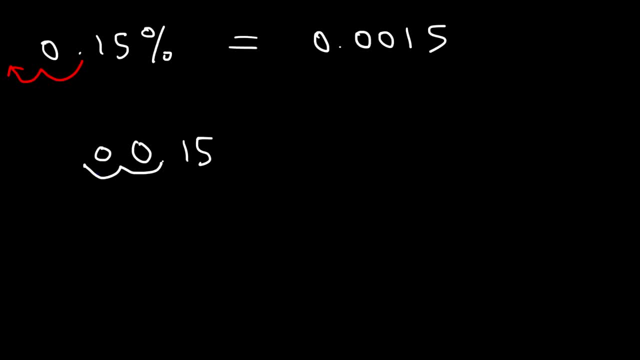 So make sure you fill in another 0.. So the decimal point is now right here. So there's two 0s in front of the 1.5.. So that's .15%. So if .15% is .0015,, 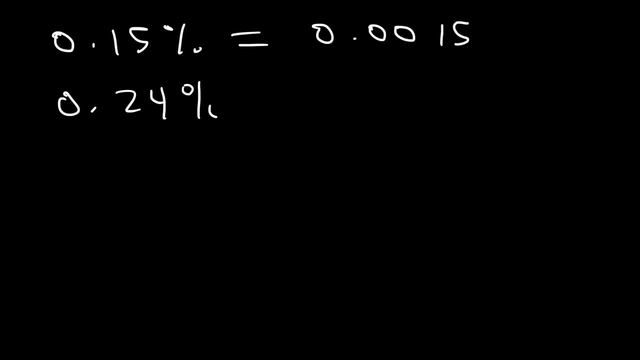 then go ahead and convert These values: .24%, .38% and .41%. So if .15% is .0015,, then .24% must be .0024.. .38% has to be .0038.. And the last one, .0041.. 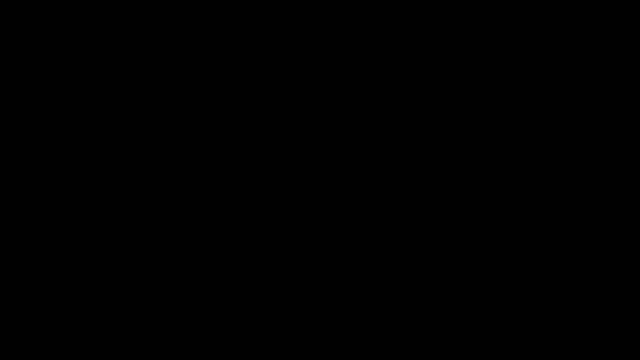 .0041.. Now let's try some other problems that have smaller values. So, for example, I'm not sure what just happened there, but let's let me rewrite that .05%. Go ahead and convert that into a decimal. 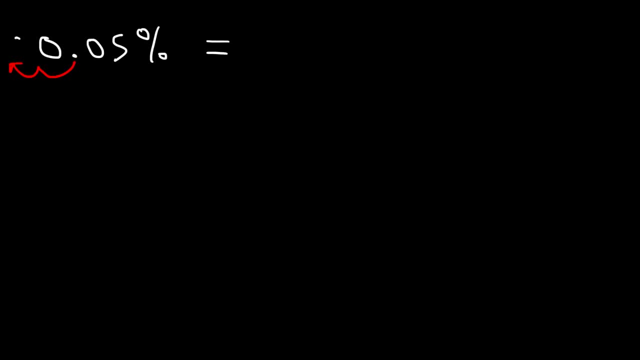 So if we move it two spaces to the left, we need to add a 0.. So this is going to be three 0s before the 5.. So it's .005.. Now try these .073%, .016% And .024% for the sake of practice. 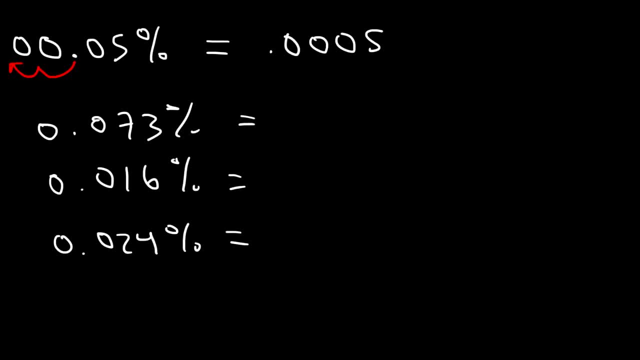 So .073%. All we've got to add is two more 0s. It's going to be .00073.. And .016 is going to be .00016.. And then this is .00024.. And that's about it. 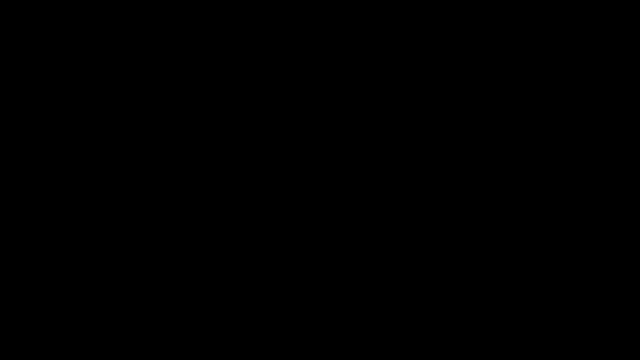 Now let's try a mixed review. Let's see if you got it. So I'm going to give you six problems and I want you to convert each percentage into a decimal. So feel free to pause the video as you work on these examples. 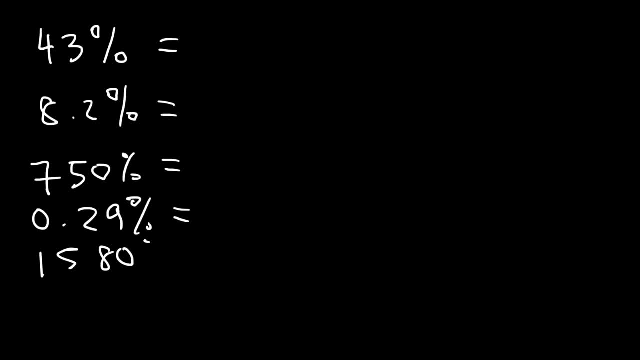 That's a 5,, by the way, Let me just rewrite that. So let's start with the first one. Let's move the decimal two units to the left, So the decimal has to be in front of the 4.. So it's .43.. 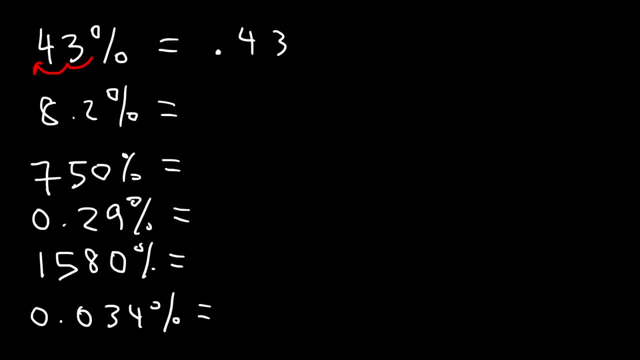 That's 43%. 8.2%. If we move the decimal two units to the left, there's going to be a 0 in front of it, 8.. So it's going to be .082.. 750% If we move the decimal two units to the left. 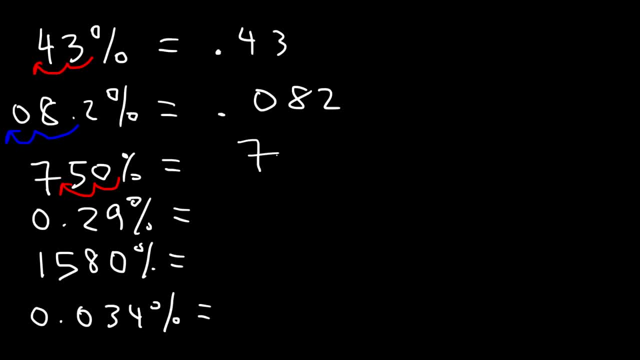 it's going to be between the 7 and the 5.. So it's simply 7.5.. Now for .29%. there's going to be two 0s in front of the 2, 9. So it's .0029.. 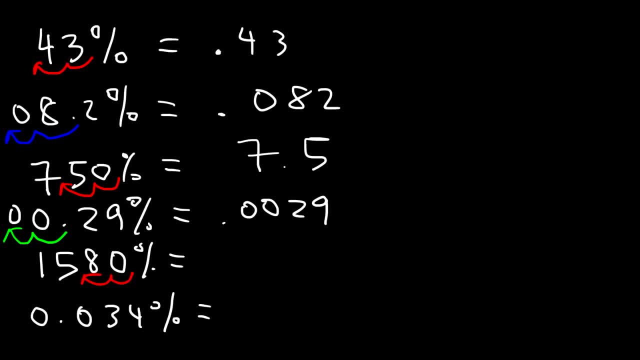 For 1580, the decimal is going to be between the 5 and the 8. So it's 15.8.. And for the last one we're going to add two 0s, So there's going to be a total of three 0s in front of the 3.. 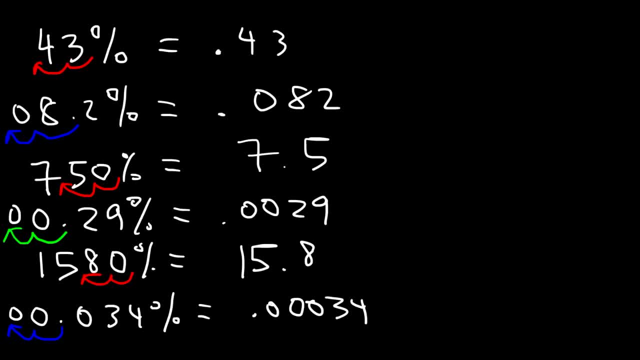 So it's .00034.. So now you know how to convert percentages into decimal values, And so that's basically it. By the way, if you want to find more videos like this, check out the description text below and you can access my pre-algebra playlist. 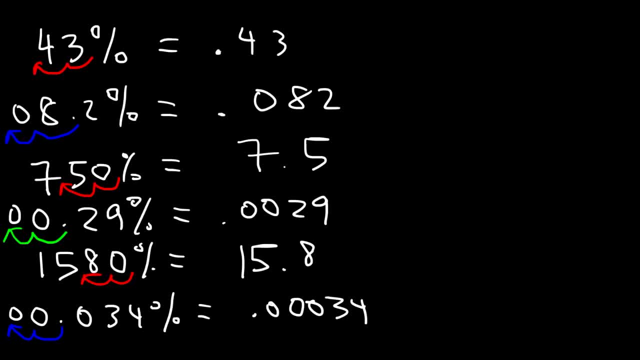 if you haven't done so already. So thanks for watching and have a great day. Now I want to show you one of my favorite things about math. This is one of my algebra courses that might be useful to you if you ever need it. 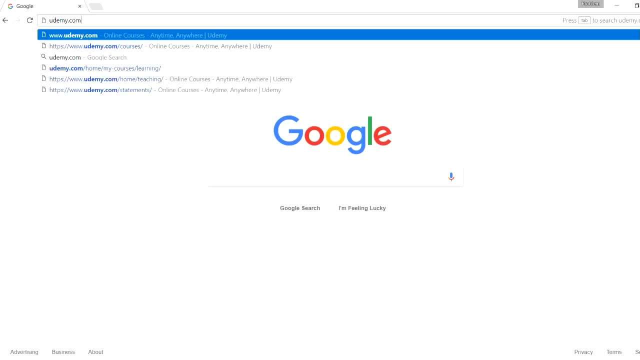 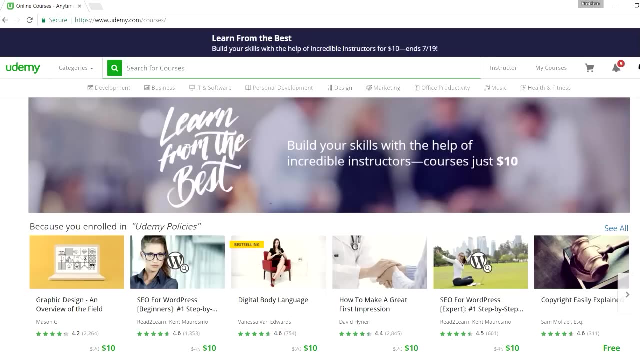 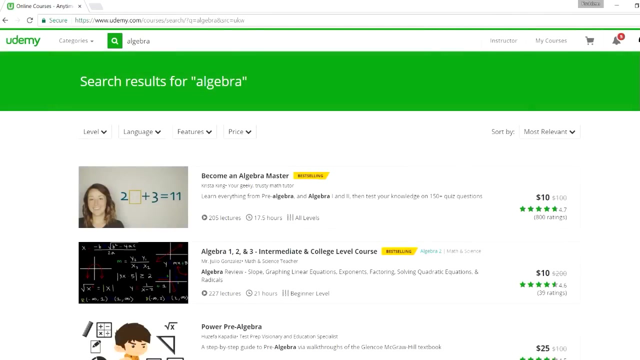 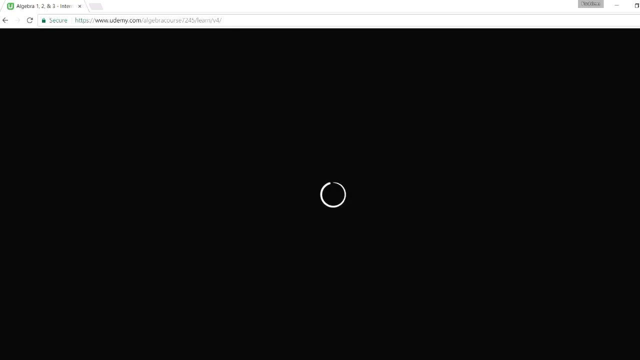 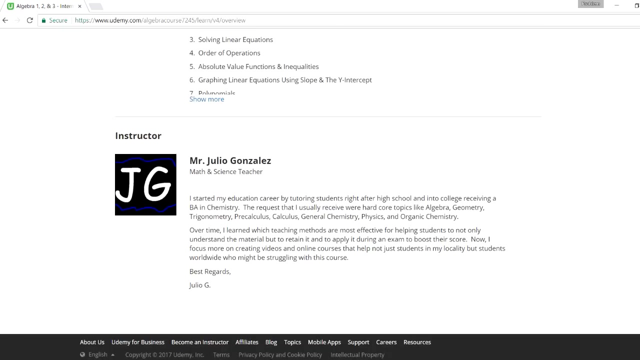 So go to udemycom Now. in the search box just type in algebra And it should come up. So it's the one with the image with the black background. So if you select that option and if you decide to go to course content, 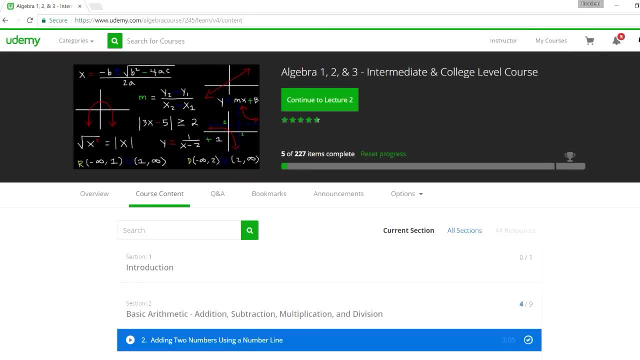 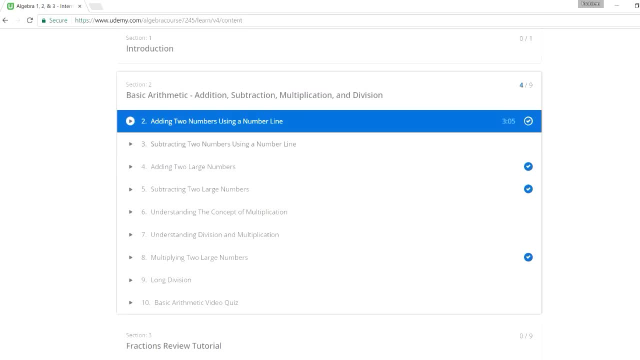 you can see what's in this particular course. So the first section, basic arithmetic- for those of you who want to focus on addition, subtraction, multiplication and division, And it has a video quiz at the end. It's a multiple choice video quiz. 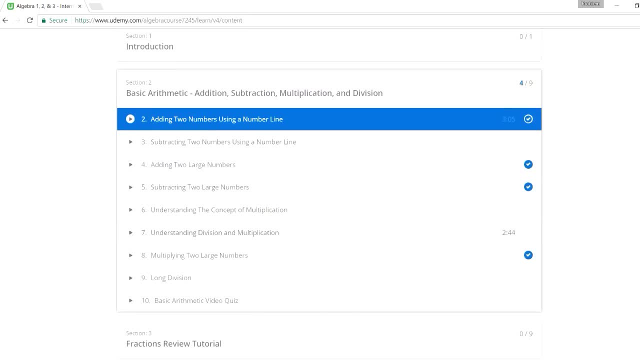 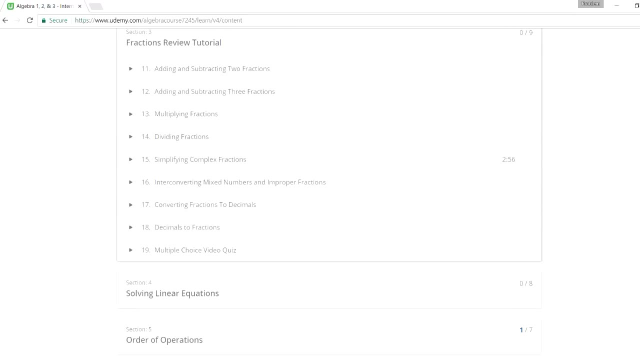 You can pause it, work on the problems and see the solutions. It covers long division, multiplying two large numbers and things like that. The next tutorial is on fractions: Add-in: subtracting fractions, multiplying, dividing fractions, converting fractions into decimals and so forth. 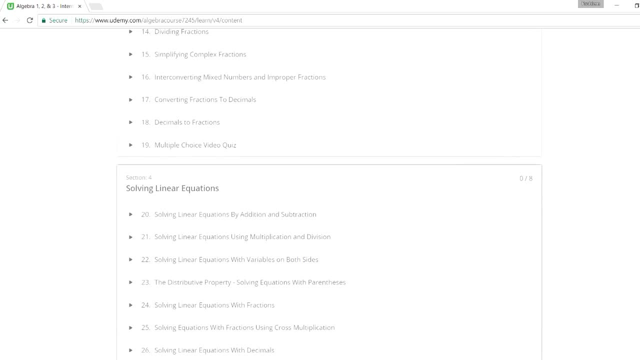 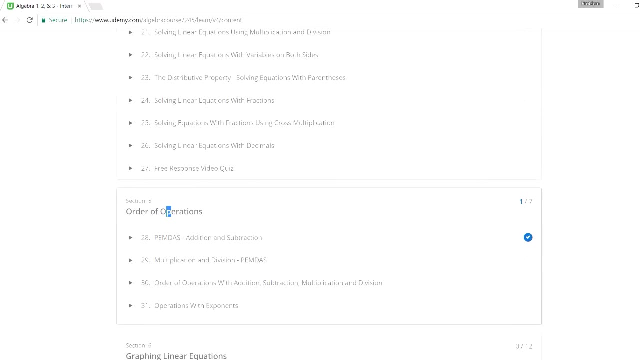 So you can also take a look at that. Next, solving linear equations, which we covered, And just more examples if you need more help with that. The next topic, order of operations, which is also useful: Graphic and linear equations. you need to know how to calculate the slope. 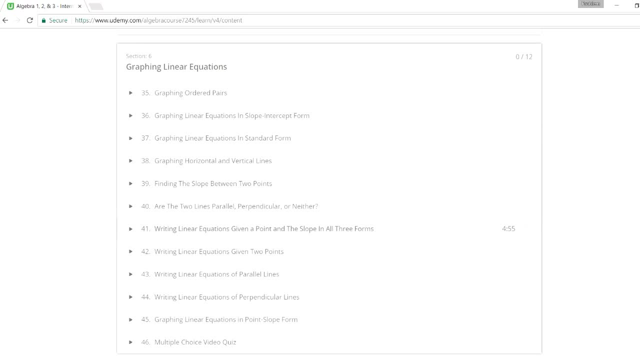 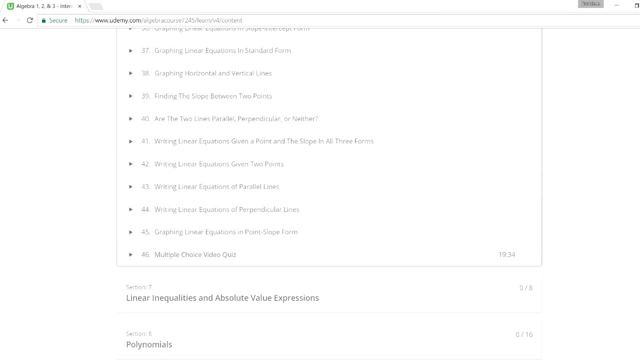 You need to be familiar with the slope intercept form, standard form and just how to tell if lines are parallel, perpendicular and so forth, And there's a quiz that goes with that as well. The next topic is on inequalities and absolute value expressions. 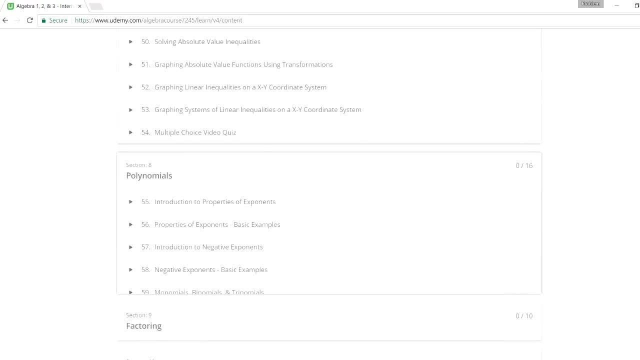 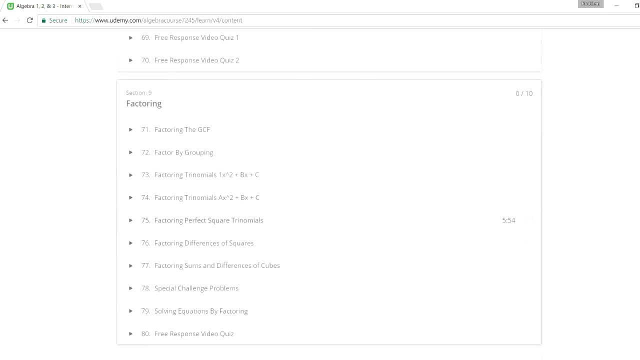 which are also seen in a typical algebra course. And then we have polynomials, and that's a long section, And then factoring you- just that's not a lot, but that's another topic you need to master- And then system of equations. 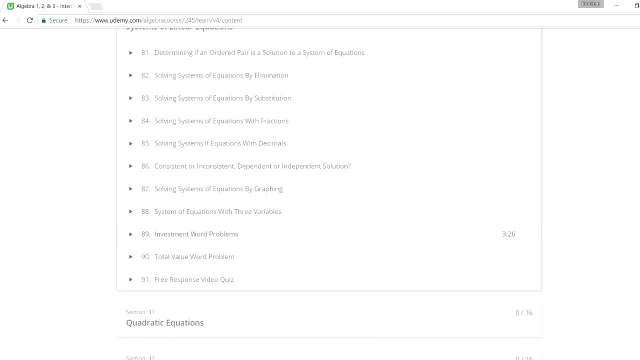 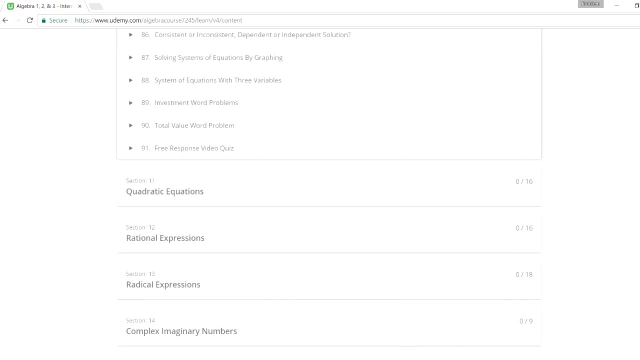 You can solve it by elimination substitution. There's also word problems as well. Sometimes you got to solve equations with three variables- X, Y and Z. So that could be helpful. Next, quadratic equations: how to use a quadratic formula.